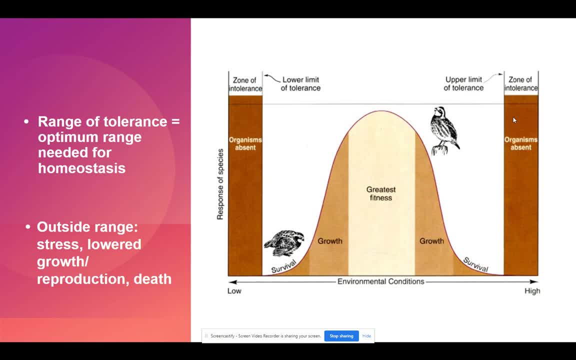 range needed to maintain homeostasis right, And there's different- you know lots of different- environmental conditions out there, But if these environmental conditions become either too high or too low, we know that that can stress out different species, And so as we get to that, 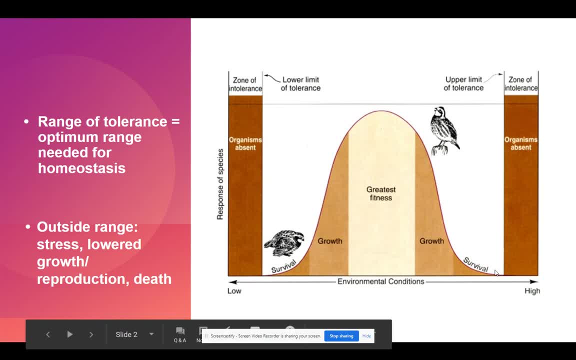 you know lower or higher level, whatever it might be, species you know become stressed out and they might experience, you know, lowered growth or reduction in reproduction and or death, right, If it becomes too high or too low, And so that's one of the things I want you to keep in mind as we look at. 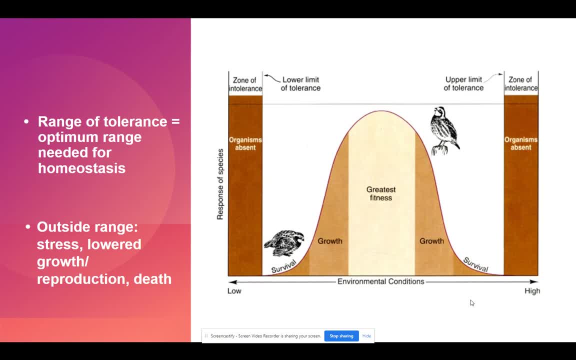 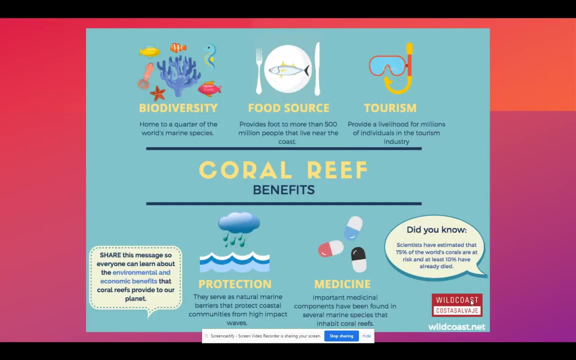 coral reefs And because there are some human impacts or some human activities that we are doing that are stressing coral reefs out and other aquatic species as well. So we're going to look at coral reefs first, though, Before we look at some of the things we're doing as humans that are stressing them out, let's point out. 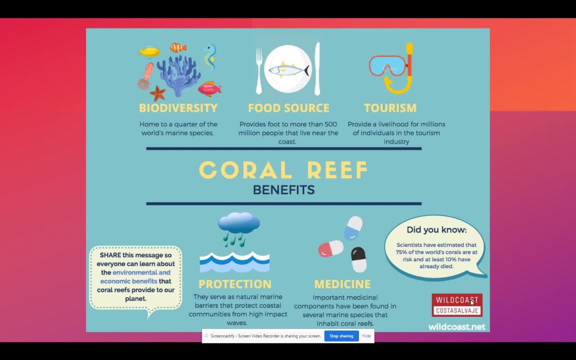 some of the things, some of the reasons why coral reefs are important. Think of coral reefs as the rainforest of the ocean. They are home to tons and tons and tons of different biodiversity. They provide us with a lot of different food, tourism, protection. 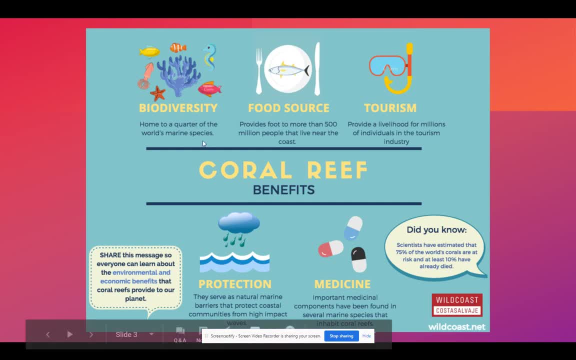 and also medicines. right, We got a little, not a fun fact, but a- I want to call it a bad or a sad fact down here. Scientists have estimated that 75% of the world's corals are at risk, and at least 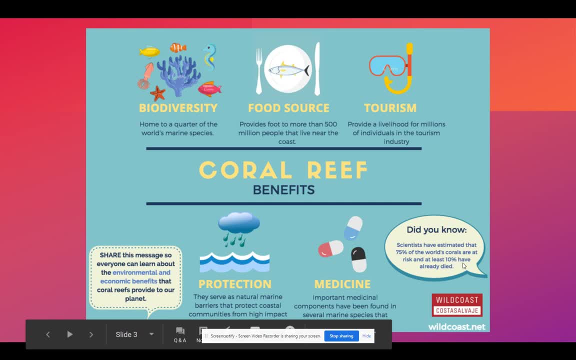 10% have already died. So we're going to look at some of the things that have led to this 10% and the 75%, why they're at risk and why so many have already died. okay, Here again are some of 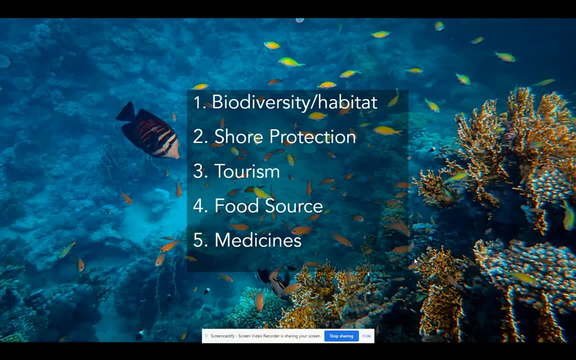 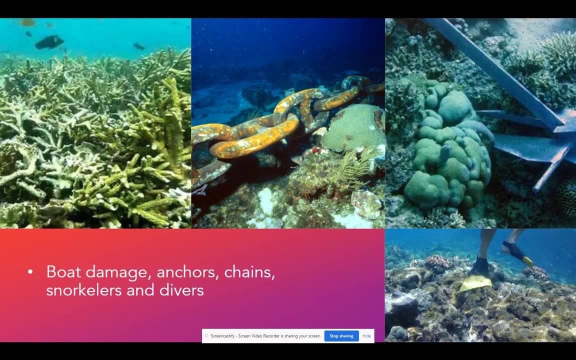 the reasons why they're at risk. So we're going to look at some of the reasons why they're at risk. Here again are some of the reasons why coral reefs are important. All right, so let's look at threats to coral reefs. Some of the more obvious threats are just like the physical threats, and that's usually. 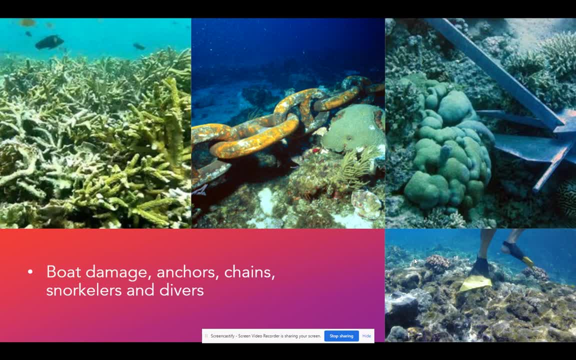 from boats, their anchors and their chains, just dropping their anchors and chains on top of the reefs themselves, and also snorkelers. as you know, tourism uh explodes in these different areas, which can be good because that, you know, helps um fund. 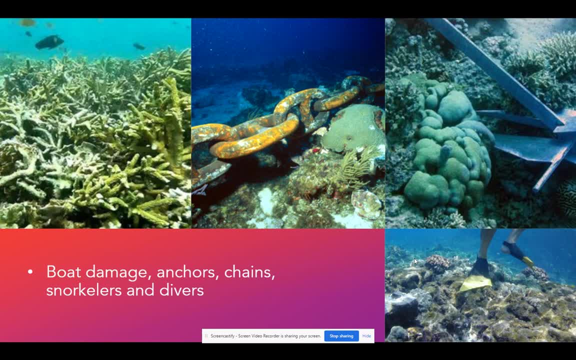 different, uh, um, different industries other than you know- fishing, And we saw the documentary racing to extinction. how you know, bringing ecotourism to different places helps, um, bring in money so that they're not, for example, hunting manta rays and things like that, right. 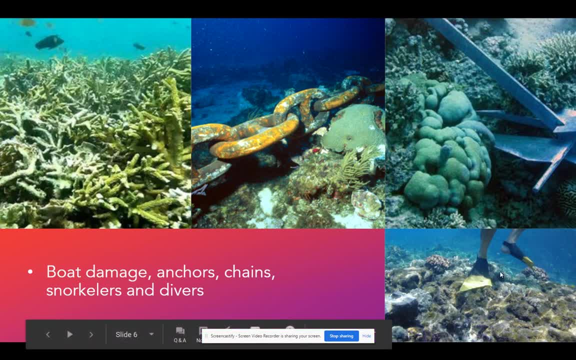 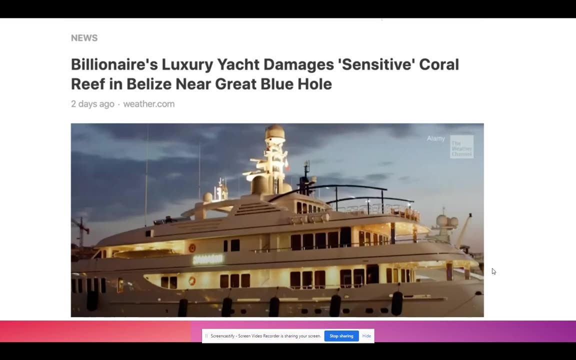 But it can lead to other issues like snorkelers damaging the reefs with their fins or touching them with their hands and breaking pieces off to bring home as sylvaneres- things like that, right. Um, here was an article about a luxury yacht, uh, damaging a reef in Belize, and this is 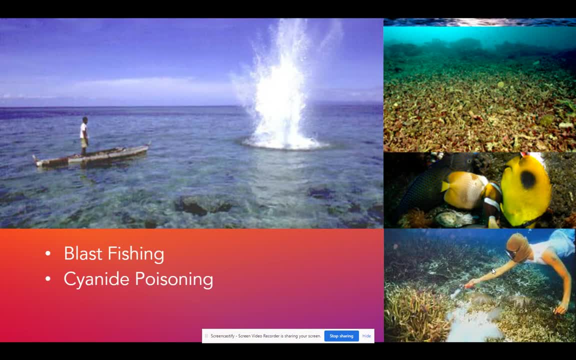 unfortunately really common Um. some other issues with physical uh threats are blast fishing, That's just the use of dynamite um to stun fish And once they're stunned they float to the top and they can be collected by the fishermen. Same thing with cyanide poisoning. 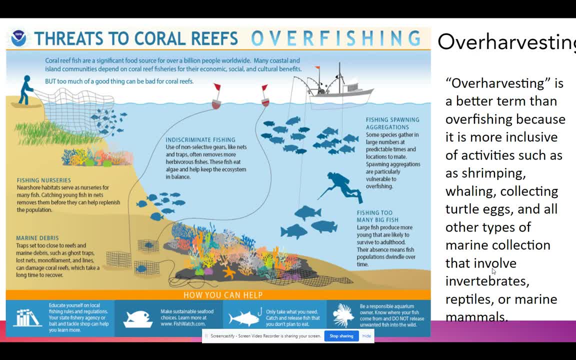 Um, and then here is just a nice infographic showing us all the different threats to coral reefs and all the different fishing styles and how they're just being attacked from all different angles And all species are are kind of at risk: Turtles. 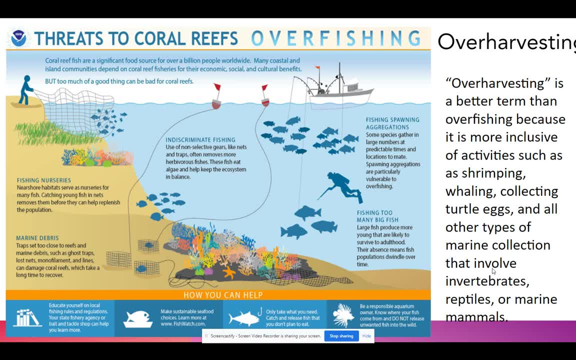 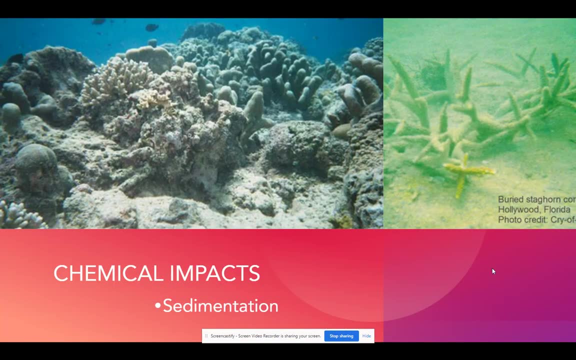 different marine life, marine mammals, uh the invertebrates, um all the shrimp and crabs and all of them are kind of being attacked from all different angles here. All the different styles of, of fishing or harvesting from the ocean. here, Uh, some chemical impacts, uh, sedimentation. 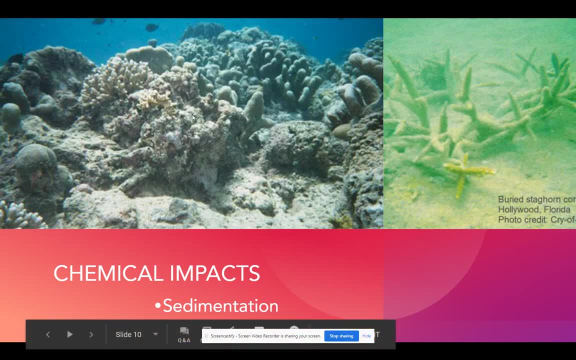 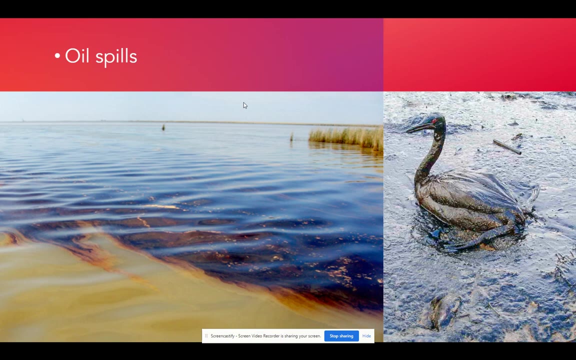 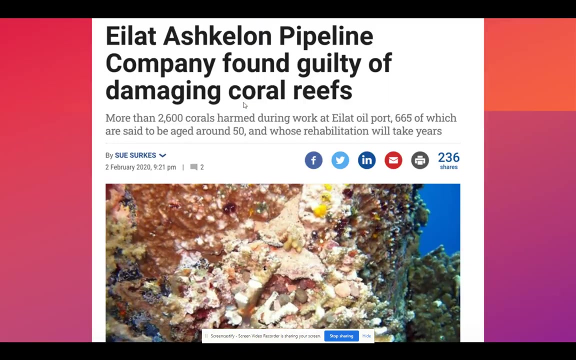 Sedimentation is just the increase in sediments from above falling and building up on these different reefs, And that usually um occurs because of the increased erosion that's happening on land. Oil spills, of course, are terrible for the marine life, and birds and all the mammals will occupy that. 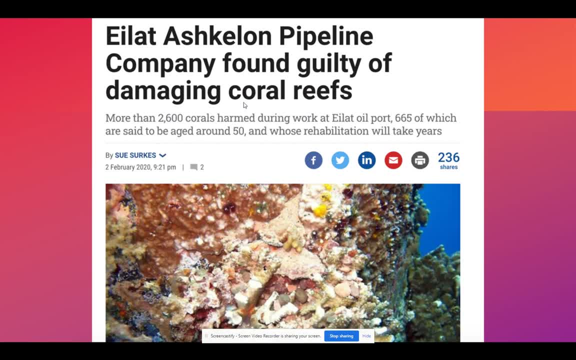 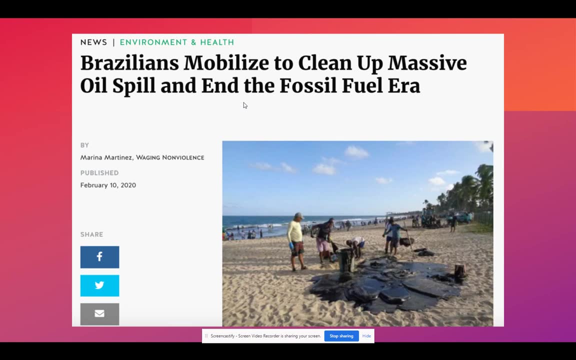 space. Here was another article in the news about a pipeline that damaged some reefs. This was in February- uh February 2nd of 2020.. Here was another recent article of uh. oil spill in Brazil, February 10th of 2020.. 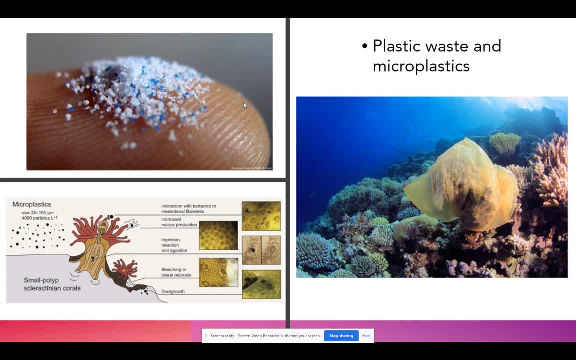 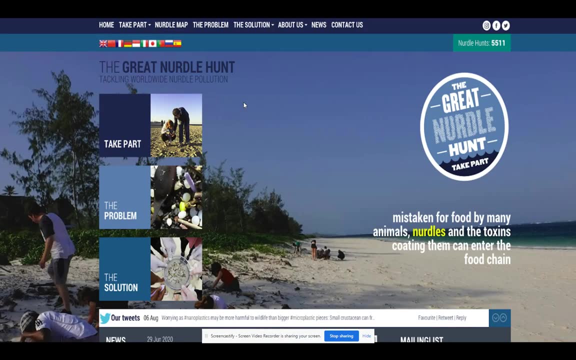 Um plastic waste and microplastics. We know that that is a major issue in our oceans- Just the amount of plastic in the microplastics that we're finding in our different marine life and um just floating around in our oceans. There's an interesting article here that we read earlier in the unit 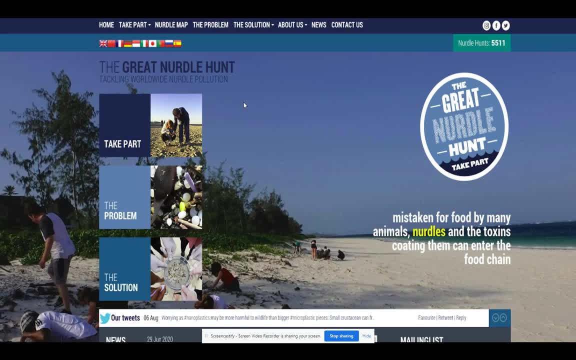 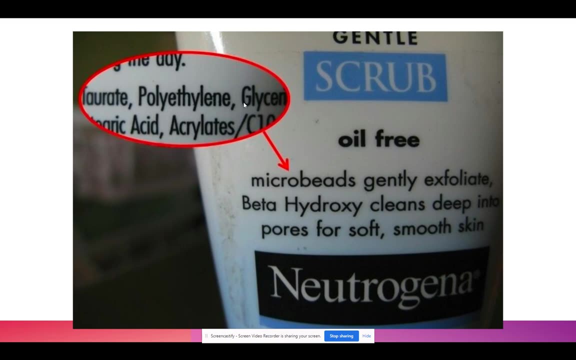 about nurdles and how these nurdles are- they're just pretty much microplastics- and how they can be mistaken um for food for many different animals in our oceans. Um, we find them in a lot of different, a lot of different forms. One um is we've all seen these face washes that have 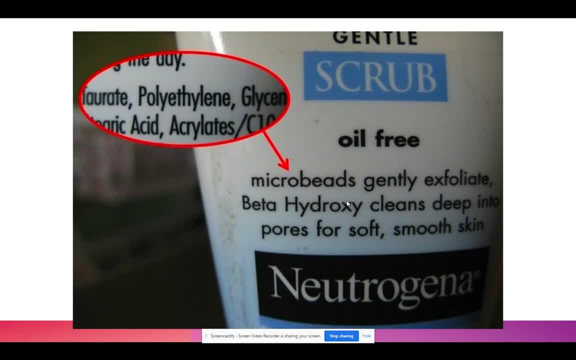 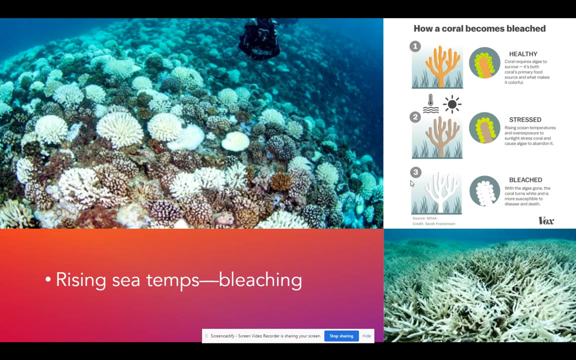 exfoliating um claims, and one of the things that they're using are these little microbeads and those that. that is an example of a uh, of a nurdle right. another uh chemical threat to coral reefs is coral bleaching and i have a short ed puzzle that i'd like you to watch that walks you through what, what coral? 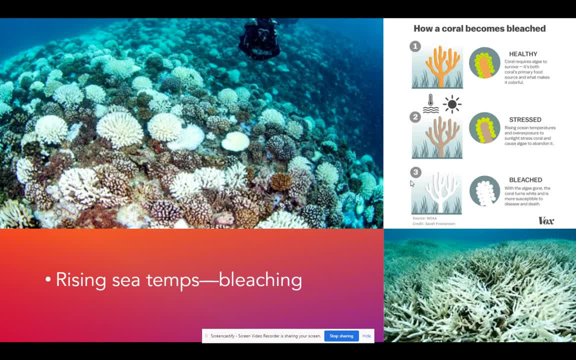 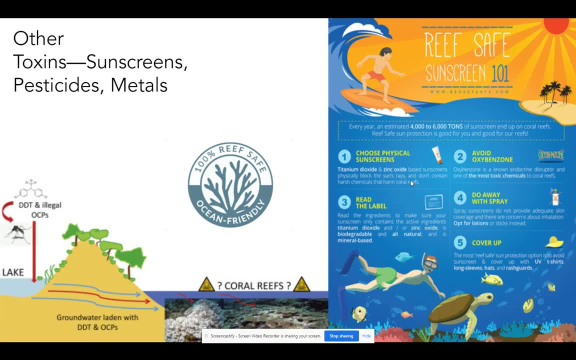 bleaching is so there's a another separate video that we'll look at to talk more about coral bleaching, um and some other toxins- that chemical uh toxins that are threatening reefs and other marine life, sunscreens, pesticides and metals. right, we know that pesticides- a lot of the pesticides that we use on land- eventually run off and make their way. 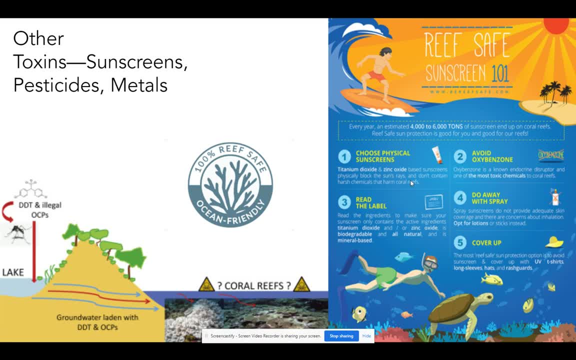 into our oceans sunscreens. even if you're not in a coral reef area, you should use coral reef um sensitive sunscreen. it doesn't have the chemicals because eventually those- those chemicals and sunscreen- make their way into our water supply and eventually will damage coral reefs in uh over a longer period of time. so just in general, we should all use. 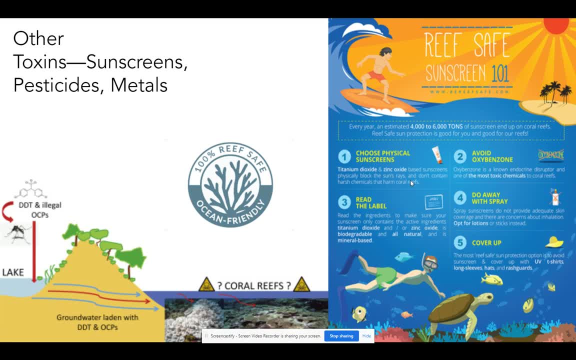 a reef safe or ocean friendly sunscreen, and they will have this stamp on them if they are ocean friendly. so when you're buying sunscreen, buy sunscreen that is ocean friendly. not only, not only is it ocean friendly, but it's also um human friendly, right. so it's more, it's healthier to use. 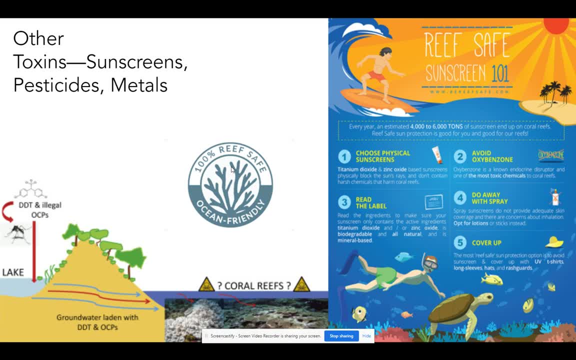 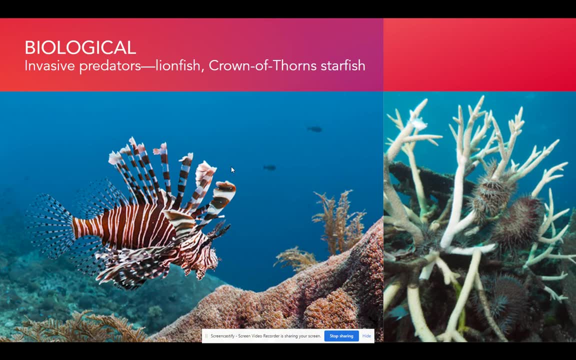 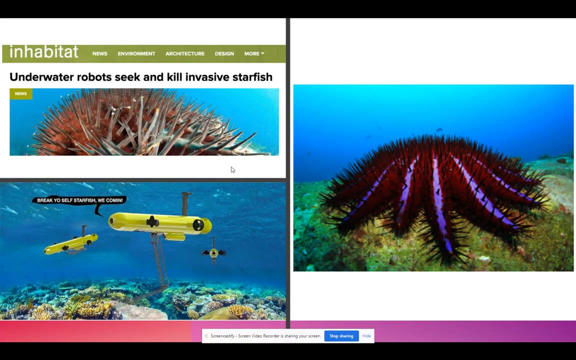 ocean friendly sunscreen compared to other sunscreens that have other chemicals in them. so read the label. all right, so some other threats to coral reefs, uh invasive species like lionfish and the crown of thorns starfish. Here was an interesting article that I found how they're using underwater robots to seek and kill invasive starfish. 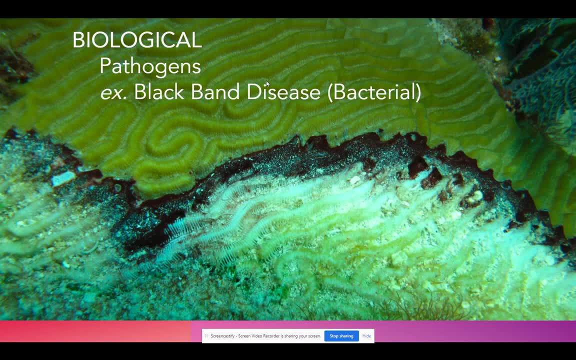 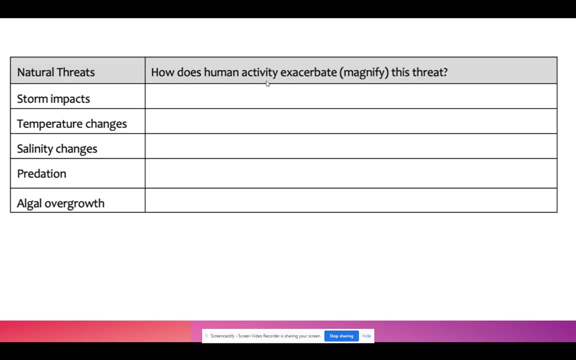 It's pretty awesome. Some other biological threats are just different diseases and pathogens that affect reefs, and these are becoming more common as the as the climate continues to change. Alright, so some natural threats that have been magnified through human activity. So storms, right Storms, temperature changes, salinity changes, predation and 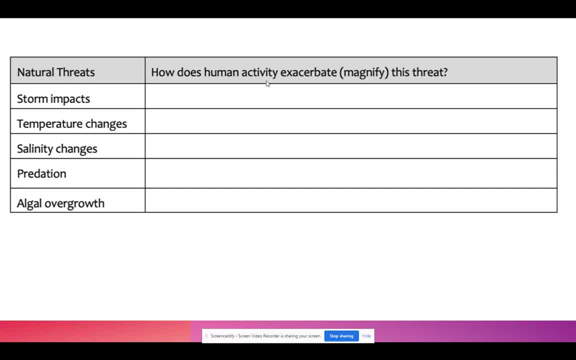 algae, overgrowth- These are all things that can threaten reefs and aquatic environments, naturally, but there's a lot of of things that we're doing that are magnifying these threats. right, and we worked on that coral reef gizmo where we looked at temperature, salinity and storm impacts, and so we know that these all 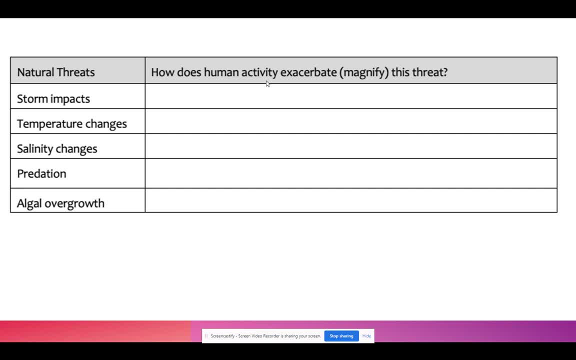 affect reefs and other marine life. here just pointing out some of the things. so storm impacts: obviously climate change. as climate change, what? what are the driving forces with climate change? we know that burning fossil fuels releases more greenhouse gases, which fuels climate change. right, so climate change would apply to all three of these storm impacts. temperature changes: 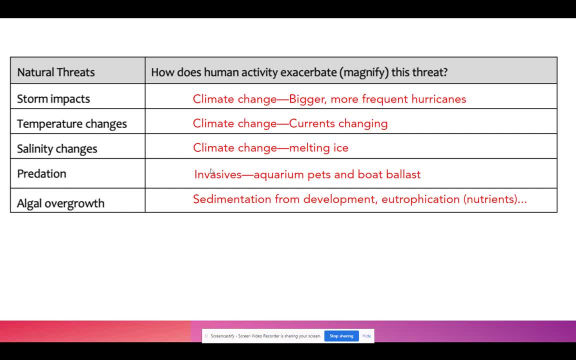 salinity changes, uh, predation, humans and our different, um you know, ships, and just human activity. we unfortunately introduce a lot of invasive species in areas that they should not be. and that's the definition of an invasive species, right. it's just a species that either gets introduced through different human activities, through 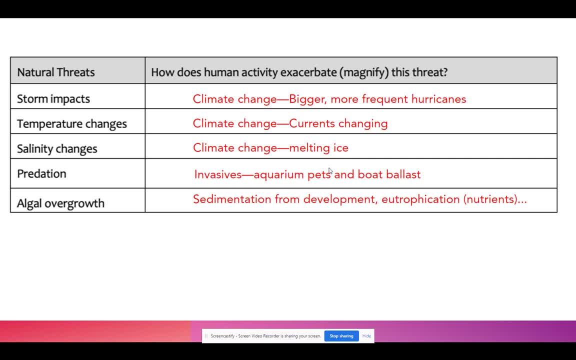 maybe it's just releasing pets or the ballast in a boat, introducing new species into environments that they wouldn't wouldn't naturally be, and then algae overgrowing growth, so just algae blooms. so we talked about algae blooms and eutrophification due to the excess nutrients in the water. so 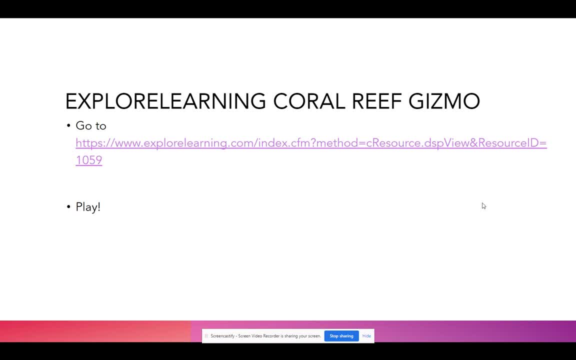 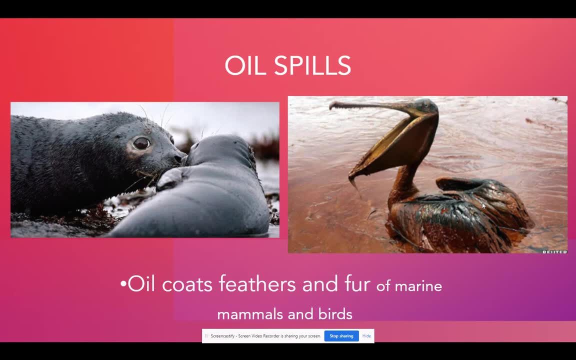 here was. we did, we already worked on this, uh, coral reef gizmo. okay, going to skip ahead to oil spills. so earlier in the week you guys watched some videos and read an article about different oil spills and we know how impactful and uh those can be on different marine life. 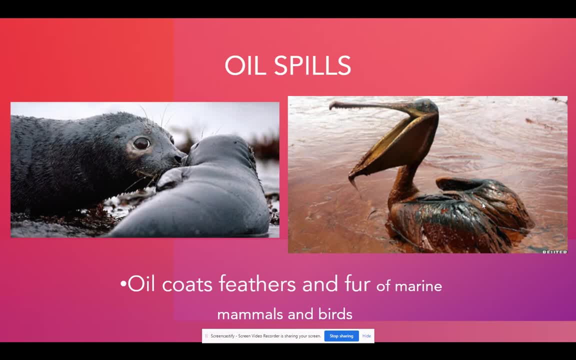 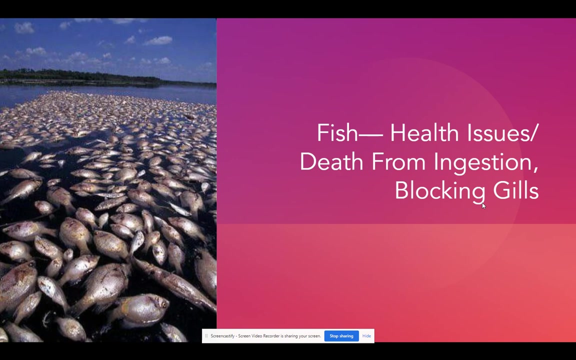 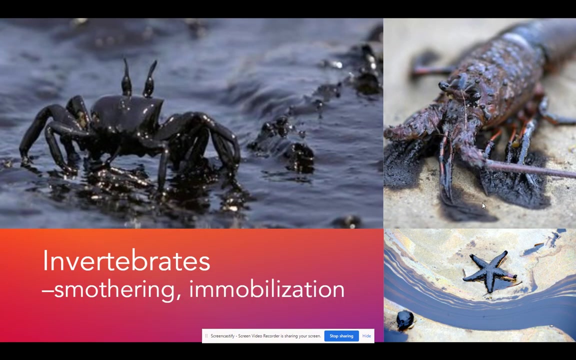 mammals, birds and all the different aquatic life. um, obviously you know the. the animals become smothered in the oil. the feathers or their fur become smothered and coated with oil. um the fish die from the ingestion of the oil. their gills become blocked, invertebrates like crabs and shrimp and starfish become smothered and immobilized and eventually die. 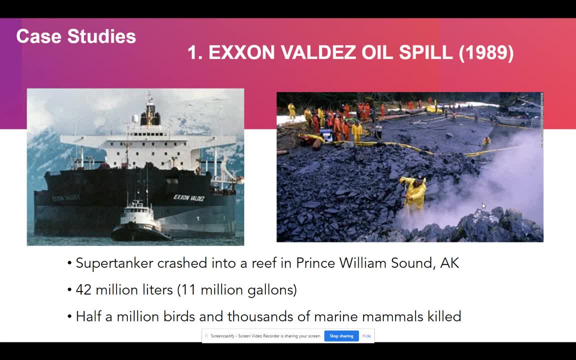 here is one case study. this was a famous oil spill in 1989. this was the exxon valdez oil spill, oil spill in in alaska, where um almost 11 million gallons of oil were released. here is a picture of that, that super tanker that released 11 million gallons of oil in alaska.